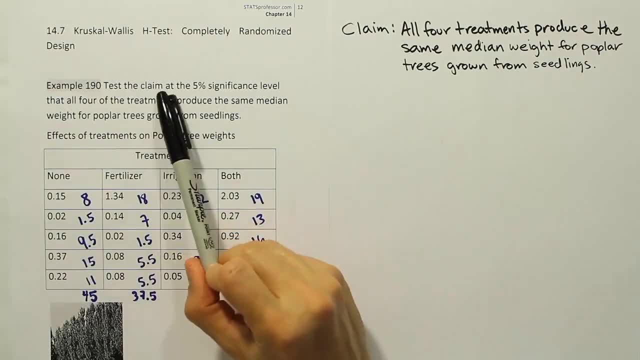 Example 190.. Test the claim at the 5% significance level that all four of the treatments produce the same median weight for popular trees grown from seedlings. Alright, so you can look at the data here and you can tell that it's a completely randomized design. 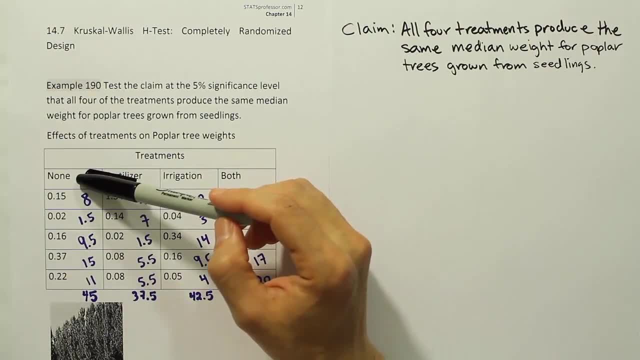 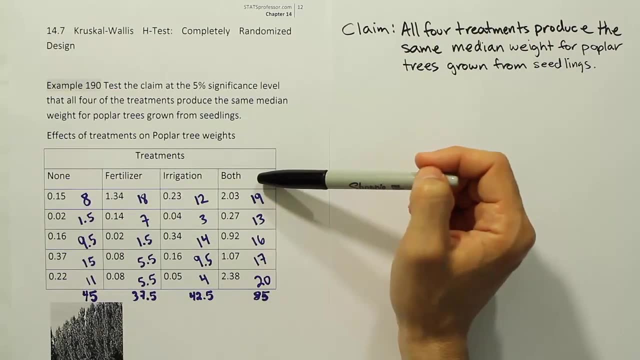 They have four treatments- They have, you know, essentially none- or a control group, A group that gets fertilizer, a group that gets irrigation, a group that gets both fertilizer and irrigation at the same time, And they're essentially four independent samples that we're looking at. 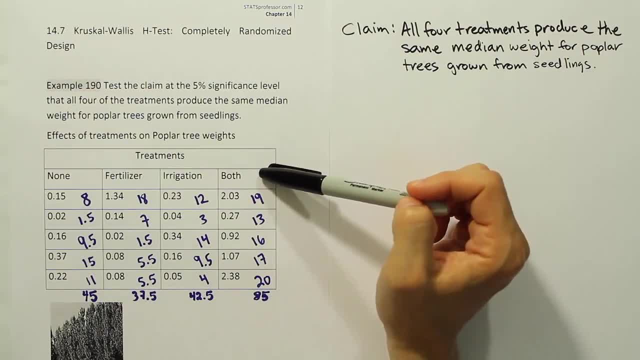 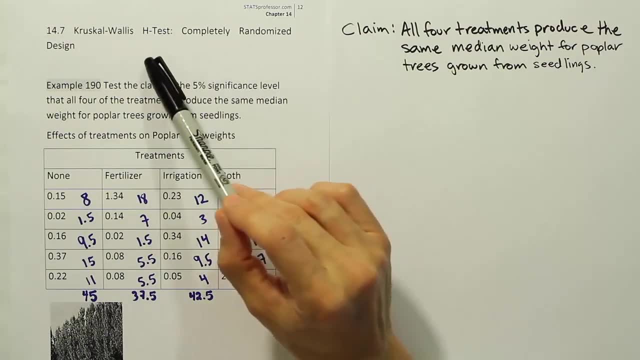 And when we do the problem, we're going to use a non-parametric procedure called the Kruskal-Wallis H-test. So this would be analogous to the ANOVA, completely randomized design or CRD experiment, But we're doing a non-parametric version of that. 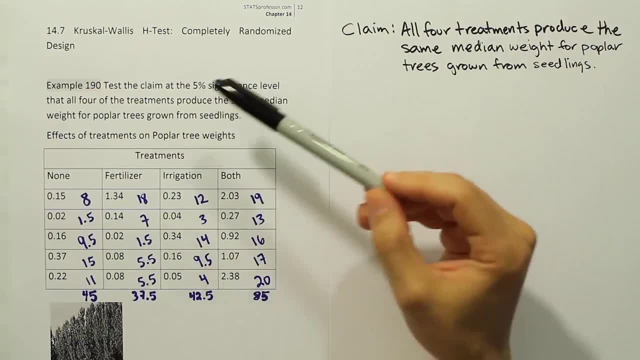 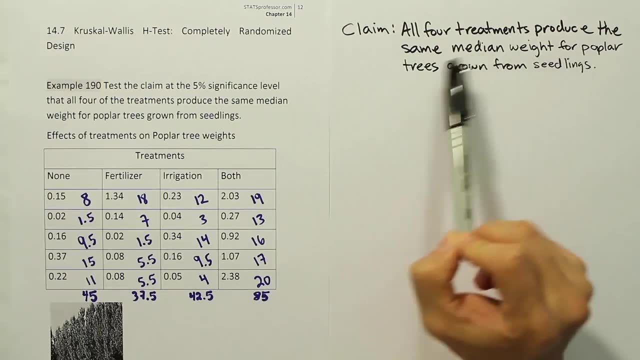 So we're going to start out with a claim, and I've already written it in here because it's just regurgitated directly from the statement here. It says: test the claim that all four treatments produce the same median weight for popular trees grown from seedlings. 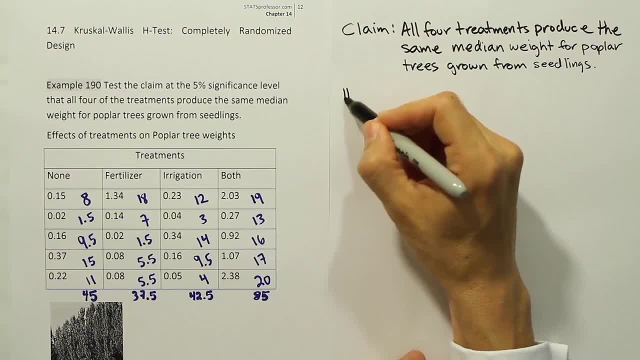 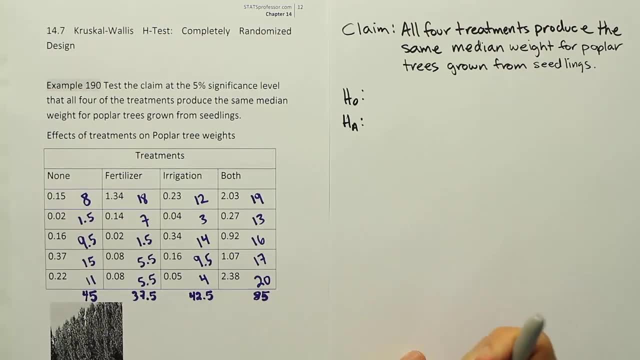 Alright, so that's our claim. But if you want to express HO and HA from that claim, we're going to use the kind of similar approach that we used in the ANOVA CRD. In other words, for these problems, the HO is always going to essentially be that all the medians are the same. 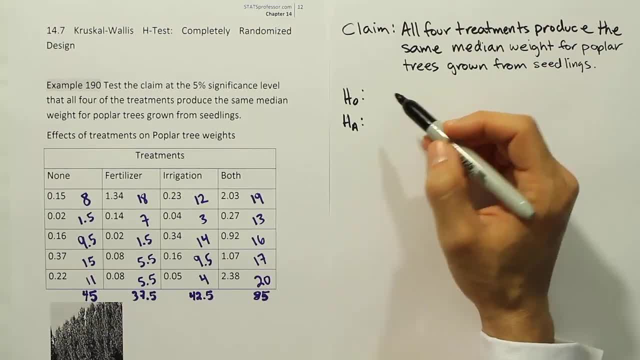 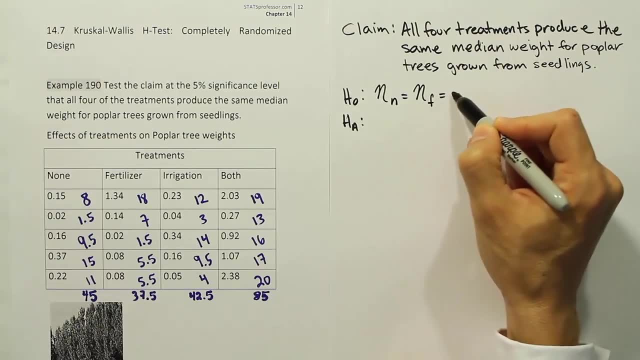 We had mean in the previous problems. Now we're going to be dealing with the median, But it's the same idea. So we'll say: hey, the median for the none group is equal to the median for the fertilizer group. It's equal to the median for the irrigation group. 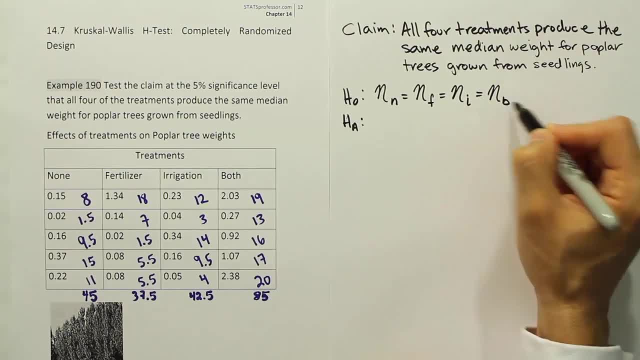 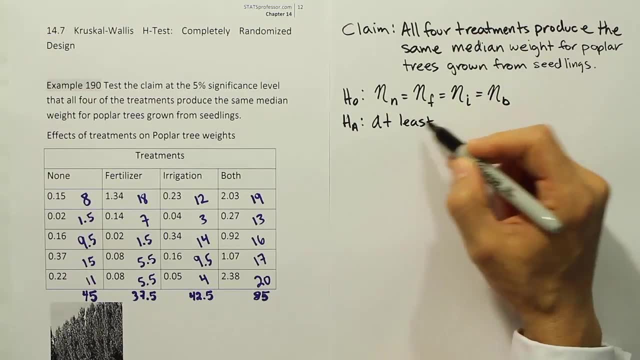 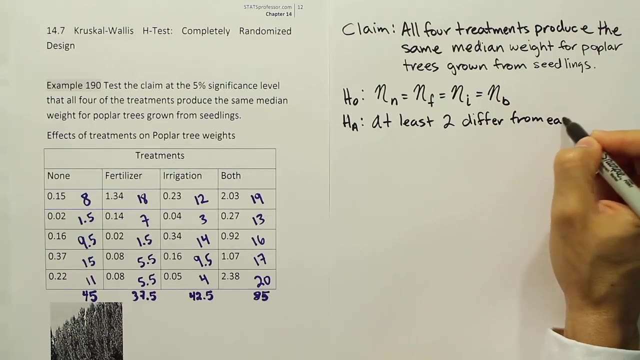 It's equal to the median for the fertilizer group. It's equal to the median for the group that uses both Right. So all the medians are the same versus at least two of them differ significantly. So at least two differ from each other. you can say from each other. 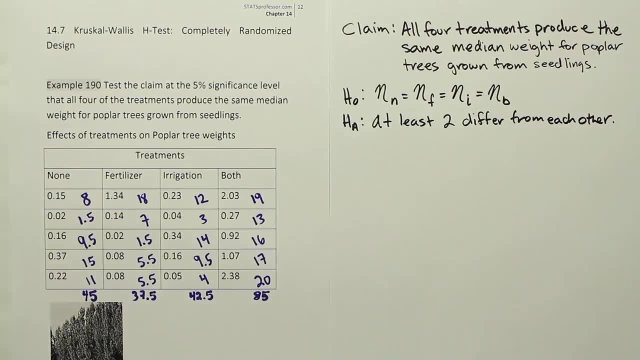 OK, so that's the same as we had pretty much for the ANOVA CRD, except we're replacing means with medians. All right Now, once we have that laid out, the next step would be to rank the data. 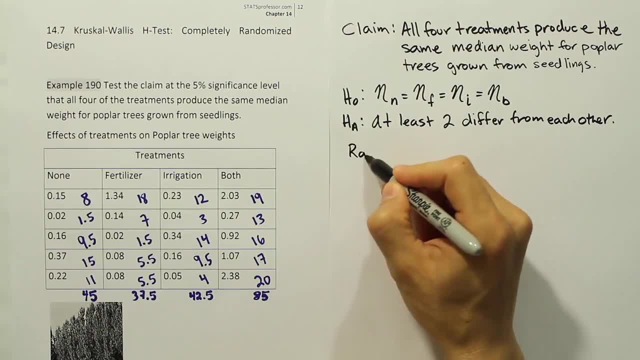 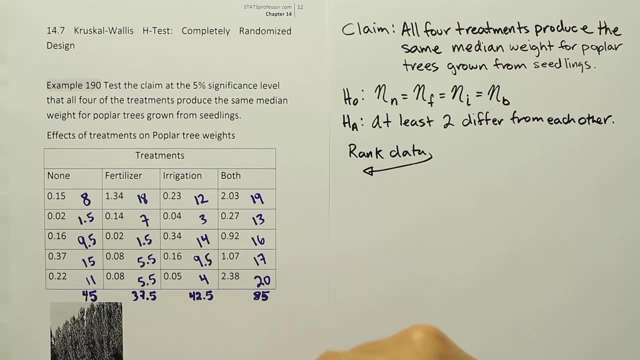 So you want to say: rank the data next. Now, I've already ranked the data and you want to rank it as if it's all from one source, Right? So, in other words, I'm not going to pay attention to these columns here as dividers. 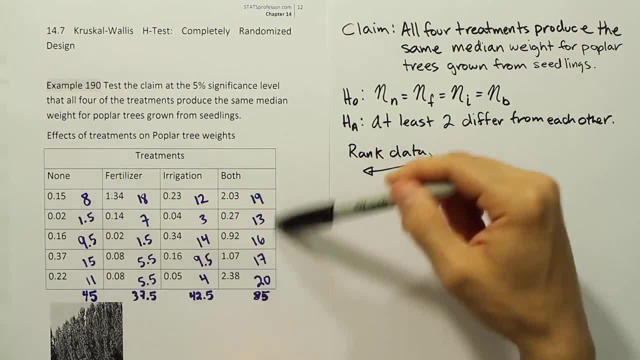 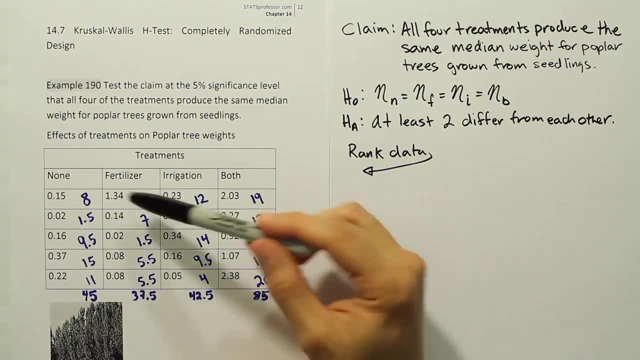 I'm just going to treat the whole sample as if it's all one big pile of numbers, and I'll rank them all according to their size. Once I've done that, though, I then go ahead and divide them up separately again into their columns. 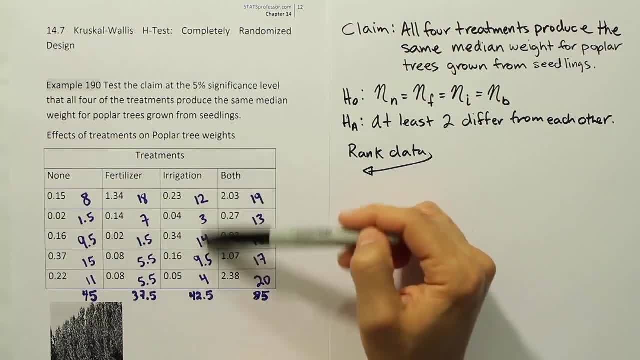 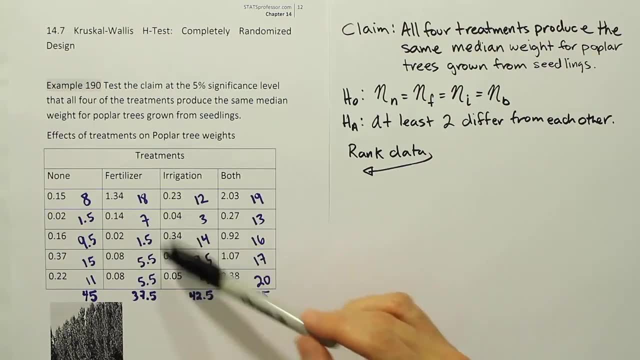 And I total the ranks in each column to come out Each column to come up with a rank total, And that's what you see that I've placed down here. I place the rank totals for each of these groups Right. So we've done ranking before. 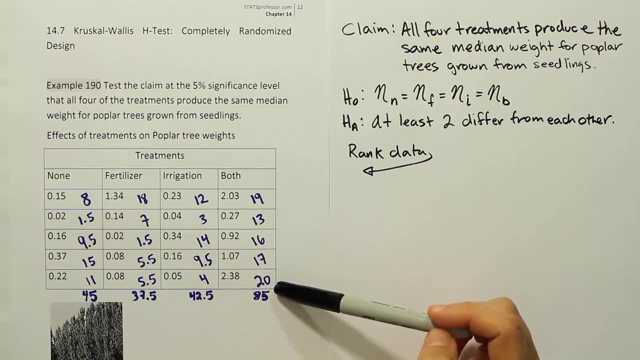 This takes a long time. So I just went ahead and do it for us, to save us some time. And then I totaled up the ranks because, hey, that's just adding And I figured you know you don't want to waste your time watching me do that. 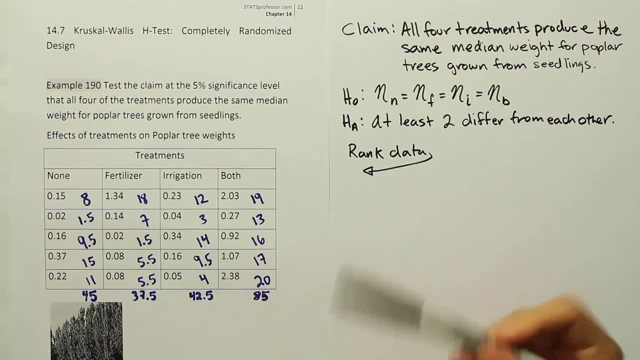 You know how that's done. But once you have all the ranks done, by far that's probably the most time consuming of this process to get all the ranks and then to add them all up. Once you have these rank totals, You're going to take them and plug them into your test stat formula. 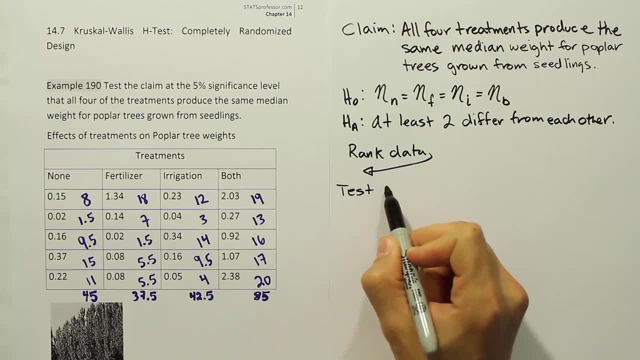 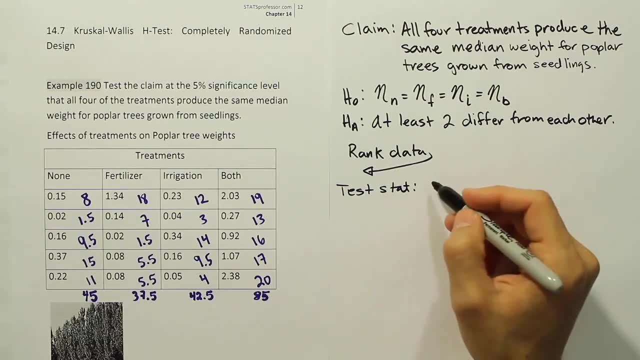 So let's write out your test stat formula. Your test stat formula is pretty complicated but it's not hard to work with. So it looks complicated but it's very easy to use. The test stat is going to be called H, That's for the Kruskal-Wallis H test. 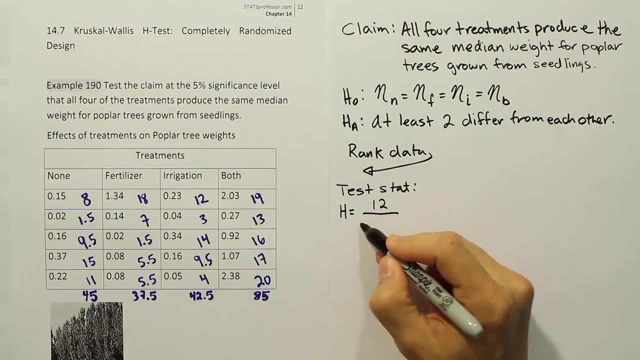 And then we're going to have 12 divided by the overall sample size, times one more than that overall sample size. Then we're going to have something that looks very similar to the ANOVA procedure When we were doing the sum of squares for treatments. 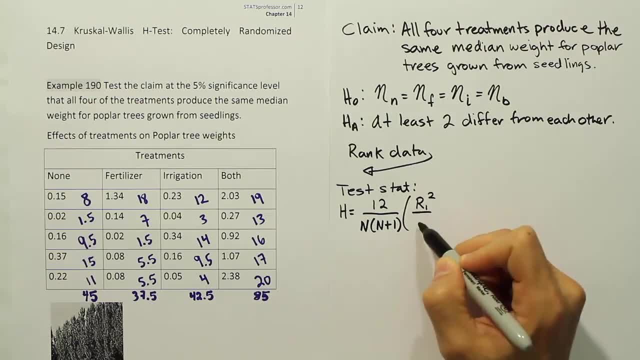 But this time it's going to be the rank totals for the first treatment squared divided by the sample size for that treatment, plus the rank total for the second treatment, squared divided by its sample size, plus dot, dot, dot. all the way down to the last treatment, or the CAFE treatment, divided by its sample size. 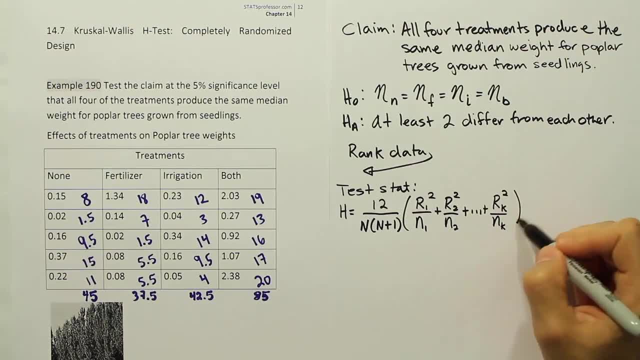 Right, All right, And then from there you're going to just subtract off three times n plus one. Okay, So let's go ahead and plug all that in now, based on what we have in this problem. So the overall sample size is just how many values we had. 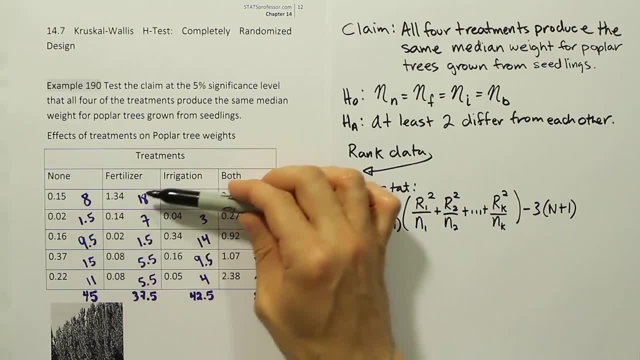 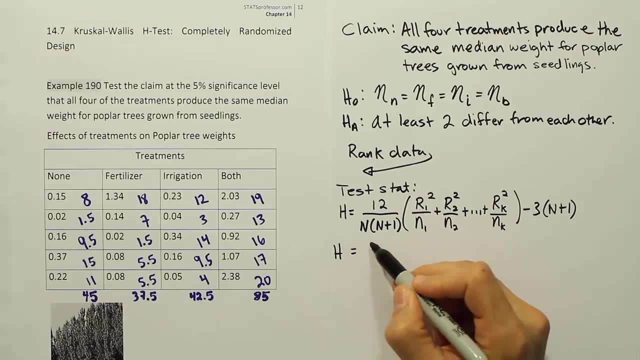 Right. So if you look at it, we have five in each of these columns. We have four columns, So that's going to be 20.. So our test stat H is going to turn out to be 12 over 20 times 21.. 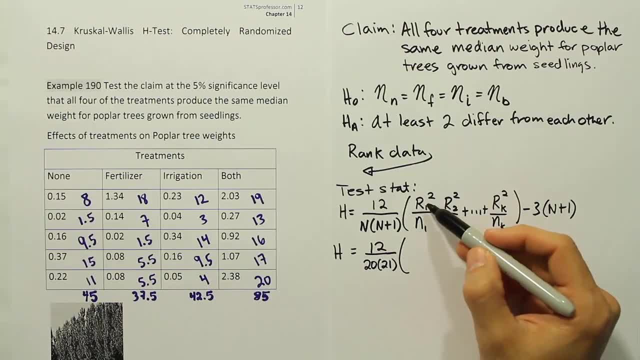 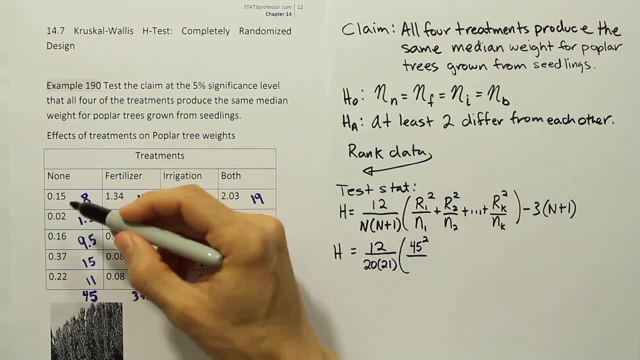 Right Times the rank total for the first treatment, which for us is 45.. Right, And then we're going to square that And divide by the number of values in that column. That's one, two, three, four, five values in the column. 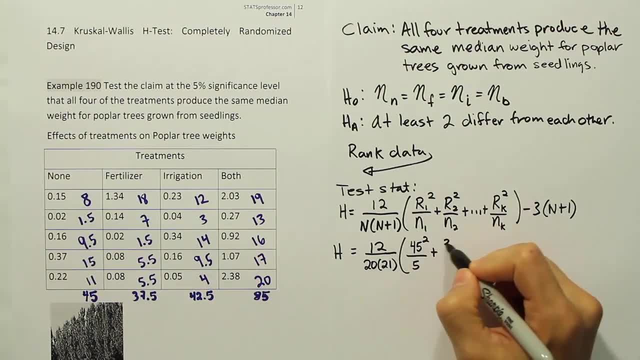 Right, Okay, And then we'll have 37 and a half squared, 37.5 squared divided by five, plus 42.5 squared divided by five, plus 85 squared divided by five. You know the logic is pretty straightforward here. 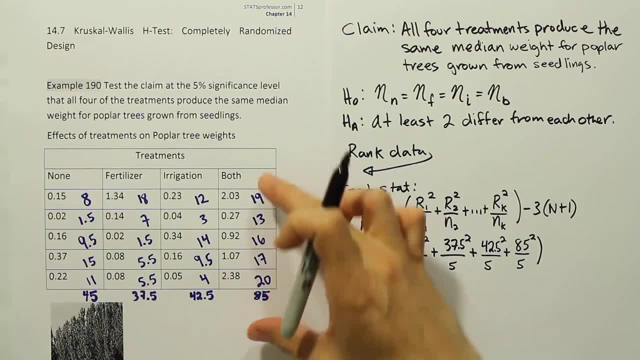 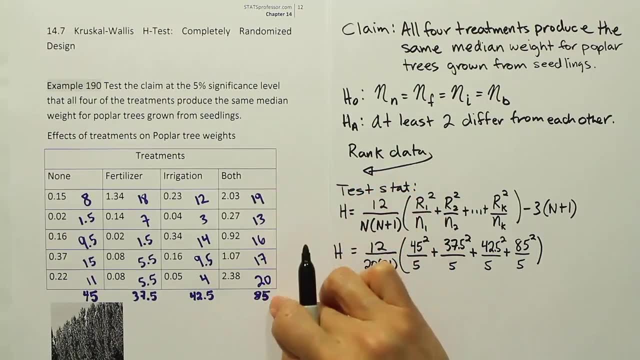 If one of these is really significantly bigger than the other, then it indicates perhaps maybe this technique has a better overall yield or produces a heavier overall weight of poplar trees Right Minus three times. So you can see this: 85, back to what I was getting at. 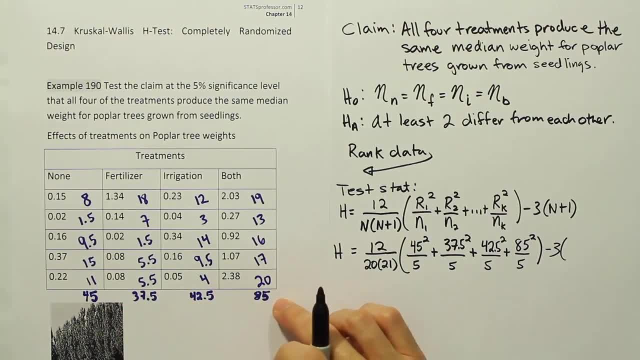 You can see this, 85 kind of stands out. That might be enough evidence to reject the null hypothesis We'll see, based on what the test out becomes Right Now. N times or sorry, three times N plus one. N plus one is 21.. 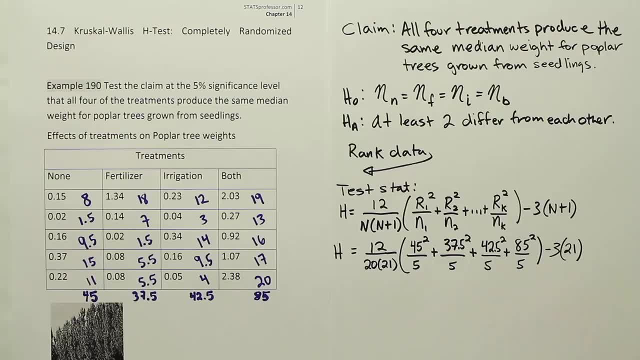 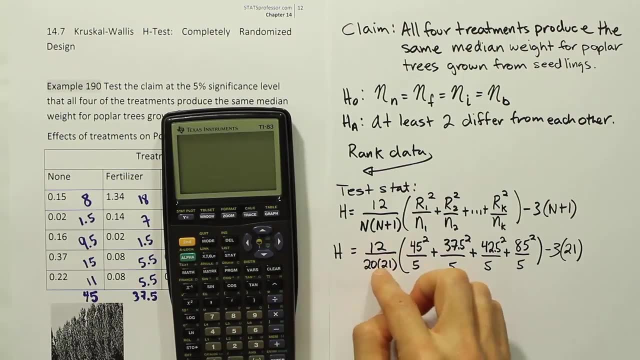 So we'll have that. All right, Let's plug that into our calculator. See what it gives us then. So we're going to have in the first part of the expression- and I want you to be careful when you do this. It's one area that a lot of people mess up on. 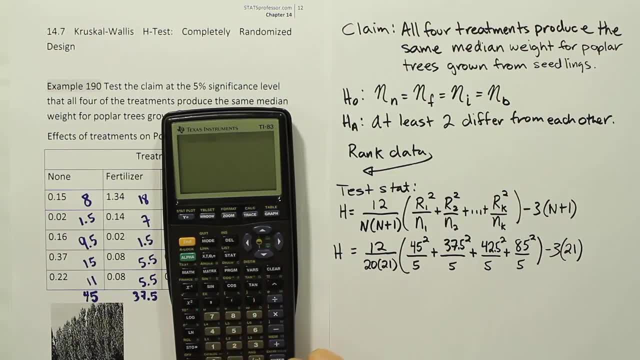 So you want to do 12 divided by- use parentheses here- 20 times 21.. Right, And then when you're done, you can either hit enter and write that out and then plug it in, or you can just take that and then multiply it by whatever follows. 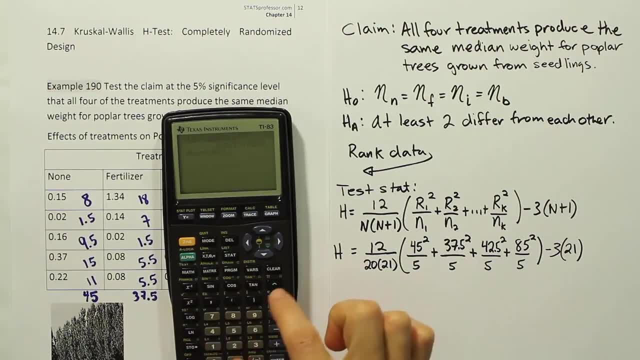 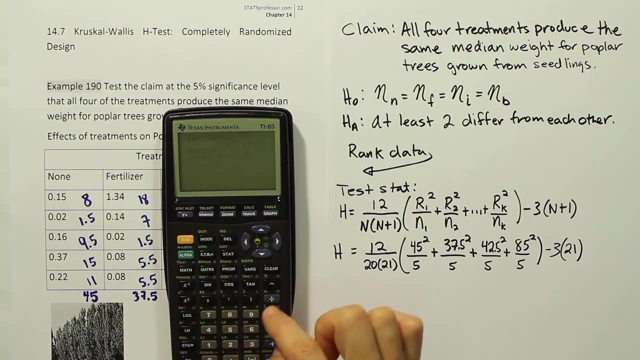 So I'm going to use parentheses. It'll have 45 squared divided by five, plus 37.5 squared divided by five plus 42.5 squared divided by five plus 85 squared divided by five. Very important, you don't make any typos here. 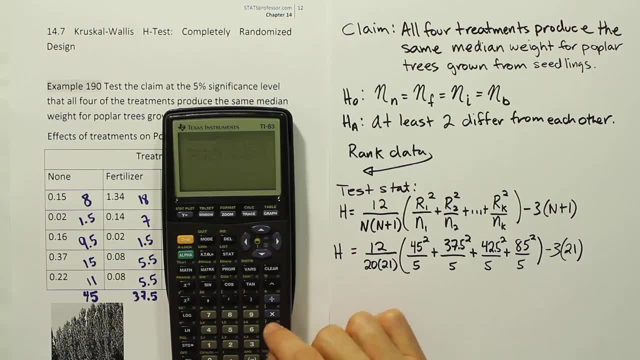 because they could be detrimental. obviously Right, It'll ruin all your hard work prior to that. Then three times 21.. So it'd be 63, or you can just type in three times 21.. Okay, When you're done, you get a total here for H. 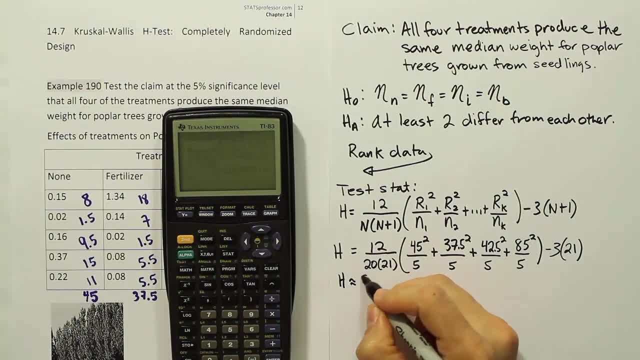 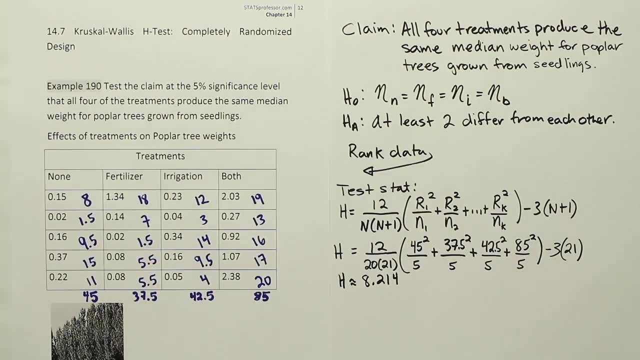 So H works out to be approximately equal to 8.214.. Right, So there is your test stat: 8.214.. Now, with that test stat, we're going to want to compare it against a critical value, Right? So how do I know if this is large enough to conclude that we should reject the null hypothesis? 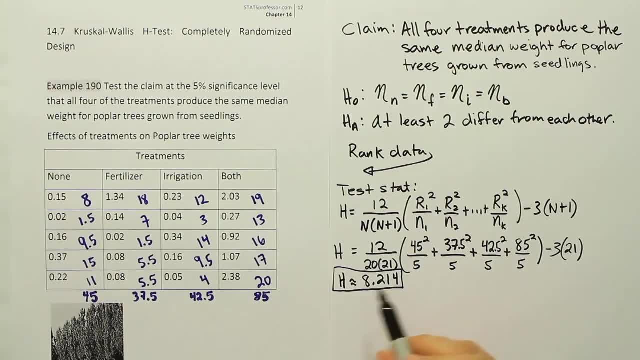 Well, the only way to know is to compare it against the test stat. It turns out that this guy has a chi-squared distribution. So when I draw my little curve as a visual aid, I'll draw kind of a highly skewed right-tailed curve. 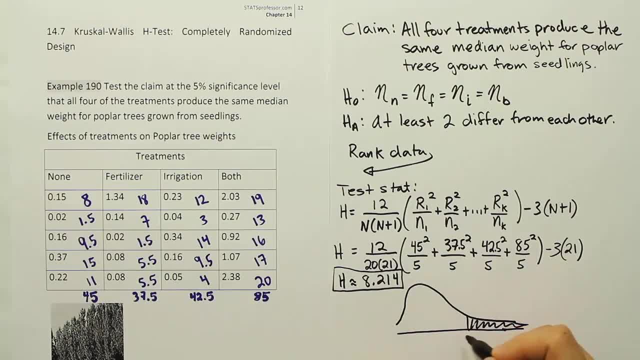 That's what the chi-squared curve looks like, Right, And then we're going to have a chi-squared critical value here. Now it turns out, the chi-squared critical value is going to have a certain degrees of freedom. First we're going to have alpha. 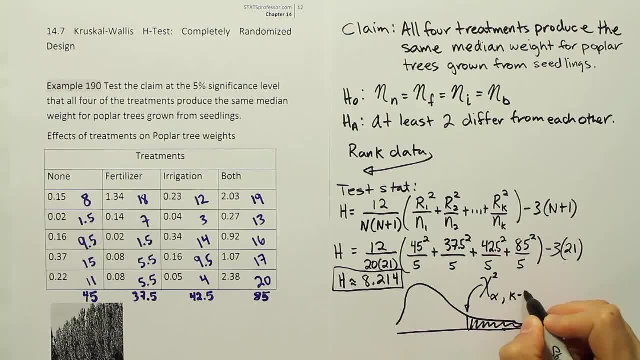 and then we're going to base our degrees of freedom on just k minus one, In other words the number of treatments that we have minus one. Here we have four treatments. Take away one, we'll have three. So for us the alpha is five percent. 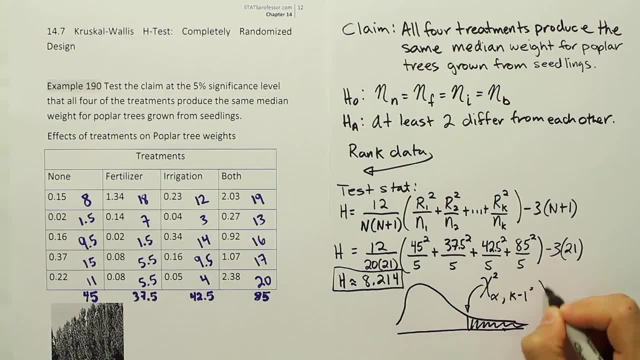 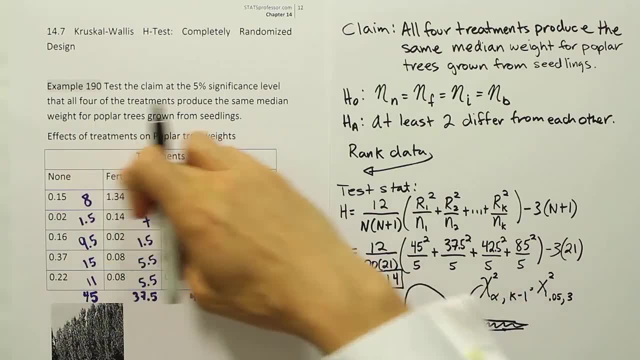 So we're going to have essentially the same as chi-squared point zero five, with three degrees of freedom, because we have four treatments. Take away one, we get three, All right, so what we need to do then is go to our chi-squared table. 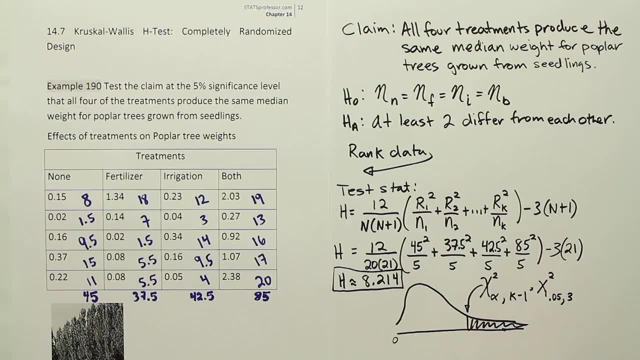 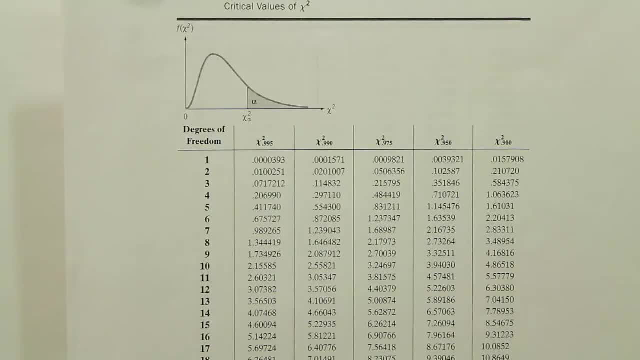 We're going to go to the point oh five column. We're going to look up three degrees of freedom and see what that gives us. Let's go do that right now. Here's our chi-squared table. We're looking for the point: oh five column with three degrees of freedom. 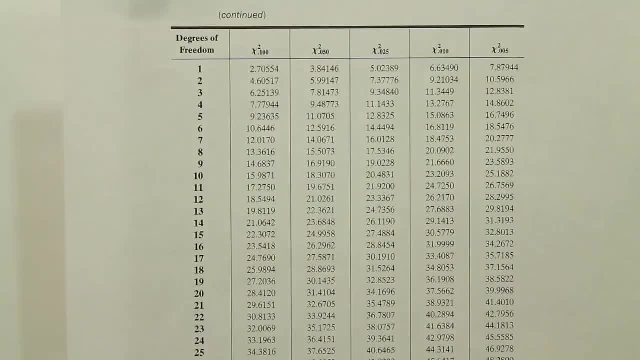 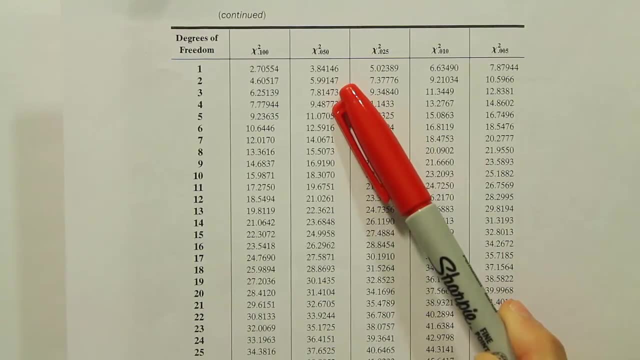 That's not any of these values. so we're going to go to the second page of the table and we find point oh five, with three degrees of freedom to give us seven point eight, one, four, seven, three. That's seven point eight, one four, seven three. 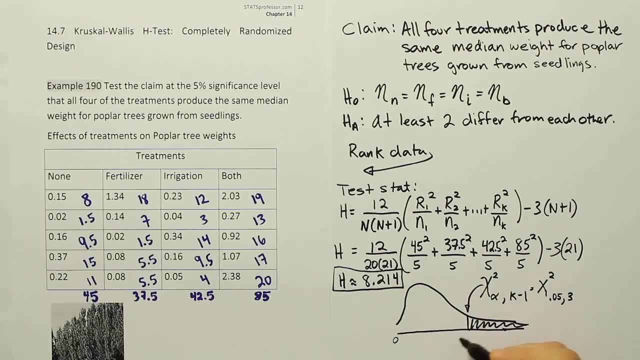 Okay, so we found the answer to be seven point eight, one four seven three. Seven point eight, one four seven three. So that's our critical value, And then from there we're going to look at our test stat. It's a little bigger right. 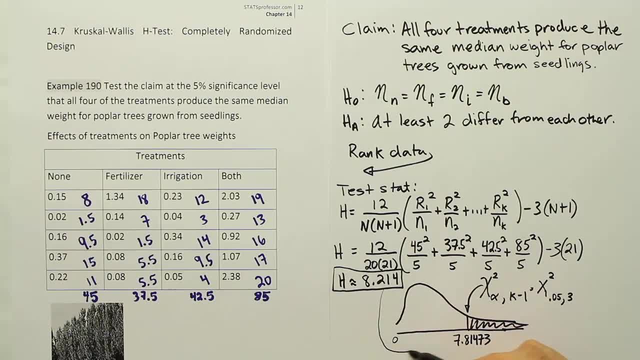 So this eight value will end up falling in to our rejection table. So we're going to end up landing over here and we're going to say that we reject the null hypothesis and therefore we support the alternative. So we reject HO and therefore we support HA.